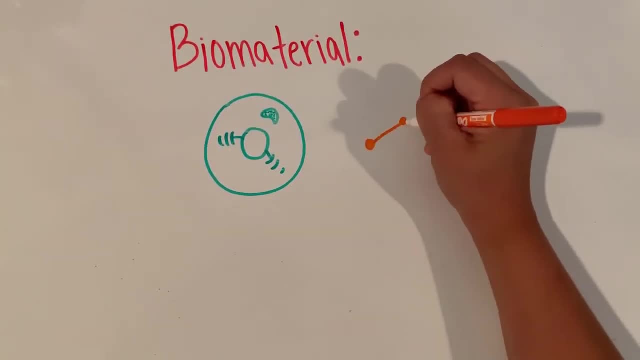 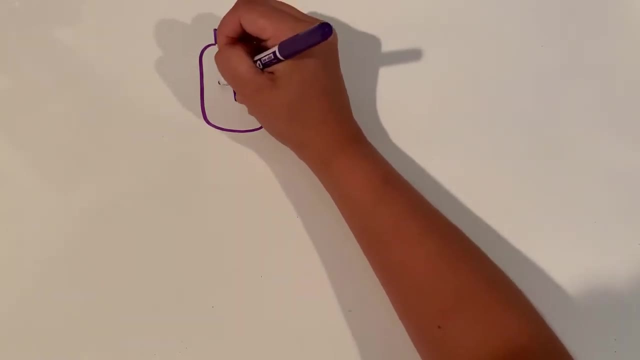 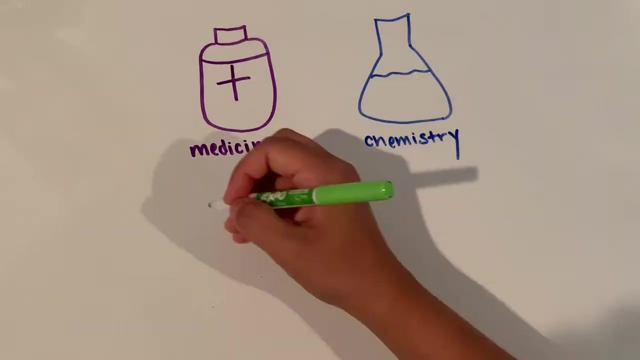 using metallic components, polymers, ceramics or composite materials- Biomaterials just like BME, and biomechanics is a multidisciplinary field that has established disciplines in medicine, chemistry, chemical engineering, mechanical engineering, biomedical engineering and material science. 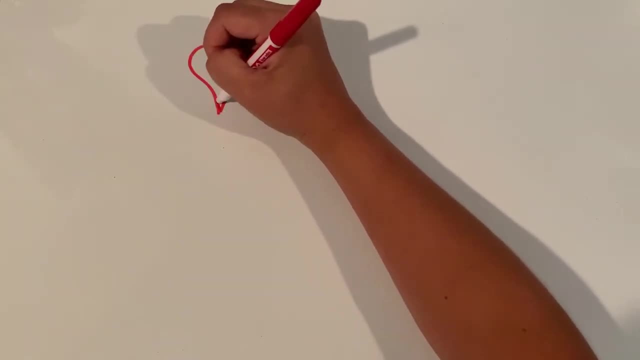 Biomaterials are used in many different ways in today's medical practice: in medical implants, methods to promote healing of human tissues, regenerated healing and active healing. Biomaterials, just like BME and biomechanics, is a multidisciplinary field that has established 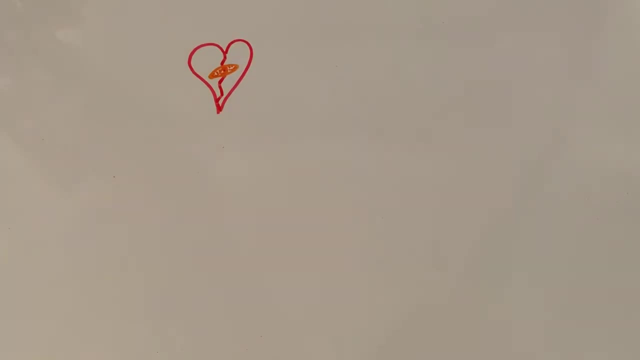 human tissues, molecular probes and nanoparticles, biosensors and drug delivery systems. Examples of medical implants include, but are not limited to, heart valves, stents, grafts, artificial joints, ligaments, tendons, hearing loss implants and dental implants. 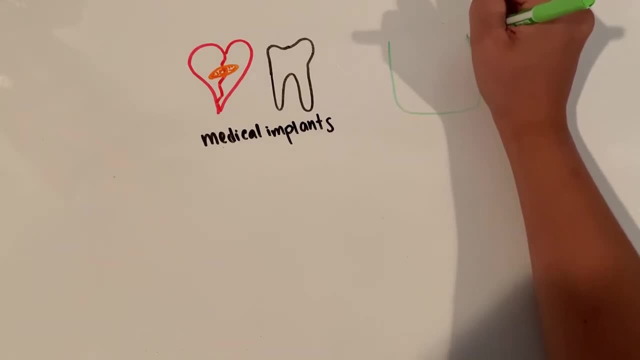 Examples of regenerated human tissues include scaffolds, cells and bioactive molecules. As far as my experience goes in this regard, I was able to spend a semester researching for the chemical and biological engineering department at RPI and got to work with BioInks. 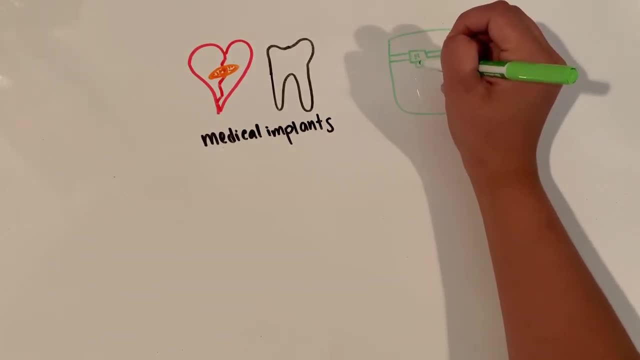 in order to 3D bioprint a human skin graft made of a matrix of different cells. The applications of such a discovery will hopefully allow for a complete healing process of burn victims, but for now, it has been established that these grafts can be used to help heal. 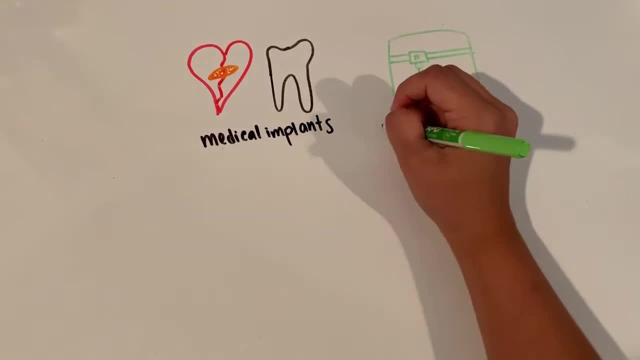 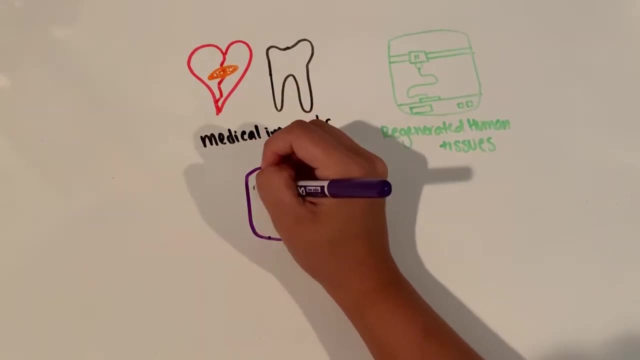 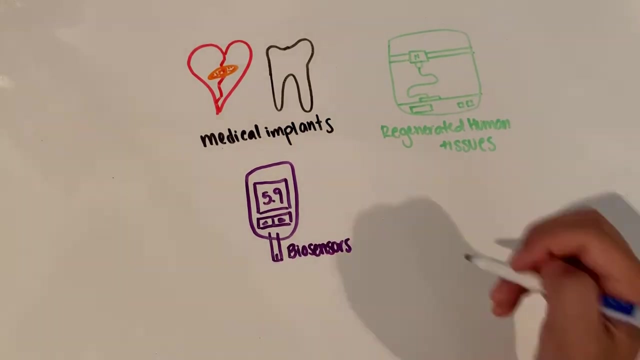 patients with pressure ulcers or diabetic ulcers as well. The definition of a biosensor is a device that is able to detect the presence and amount of specific substances and transmit the data, such as in a diabetic patient to monitor glucose levels. And finally, drug delivery systems are able to carry out and apply drugs to a targeted 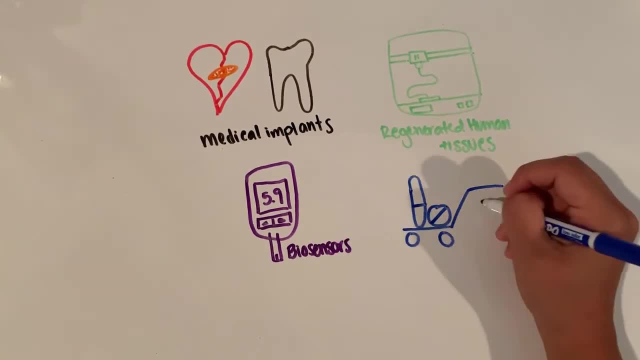 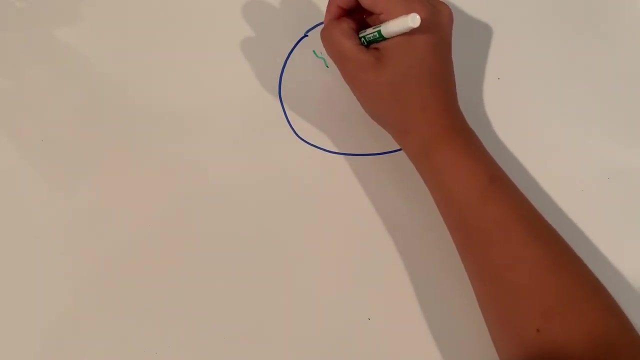 area, such as cancer patients and using drug-coded vascular stents or implantable chemotherapy wafers. Like the other two concentrations offered at RPI, biomaterials plays a role in a vast number of ways beyond what is possible today, which makes it such an integral part of society.